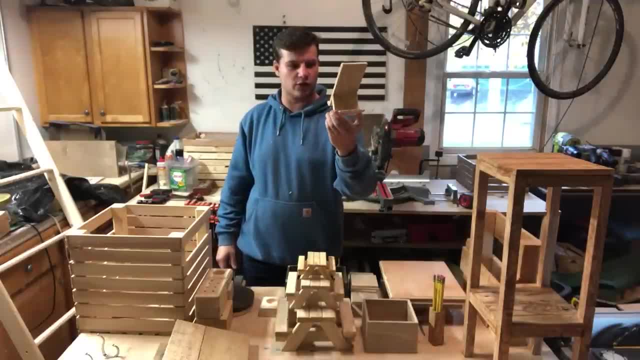 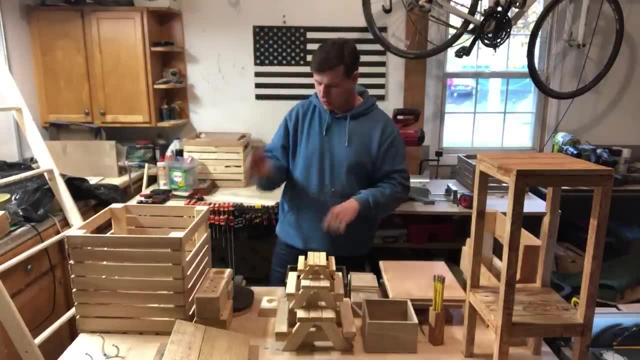 a little one that I made, putting together some scrap wood and some glue. I have the little slit right there from the charger. So that one's another great one. And then I have three other phone holder type things that I want to show you. I don't have those with me, but I would like to. 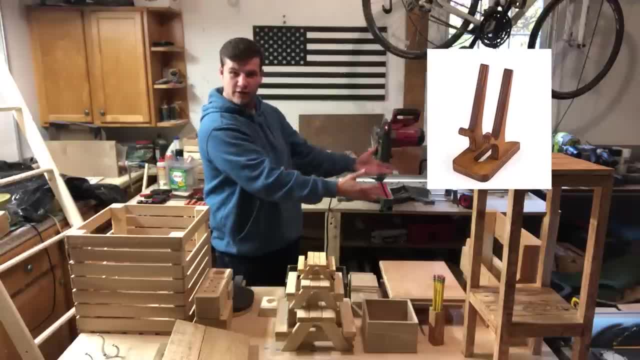 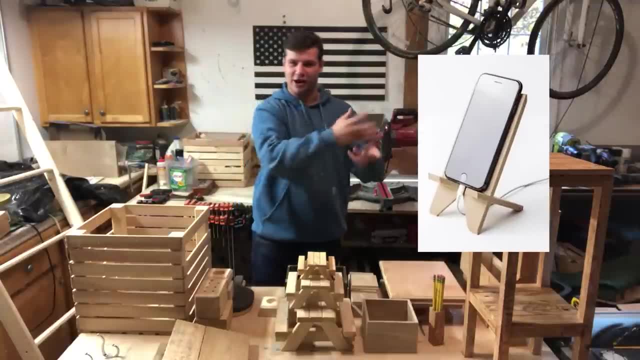 insert pictures of them here. So here's one. John, can you put a photo here? I assume This one's great, This one's also great and that one's also great. Okay, so we got three other phone holders that I have made before. I just don't have. 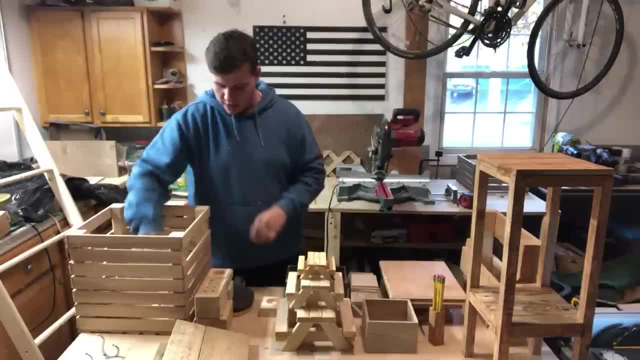 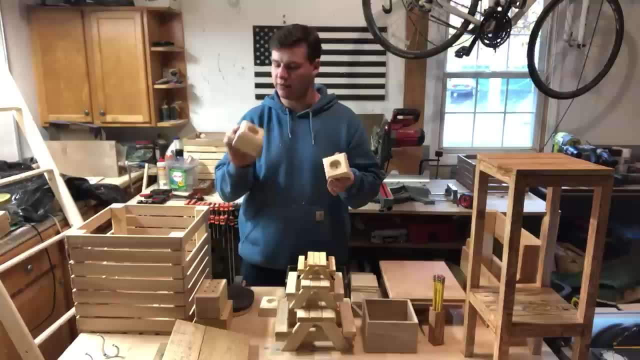 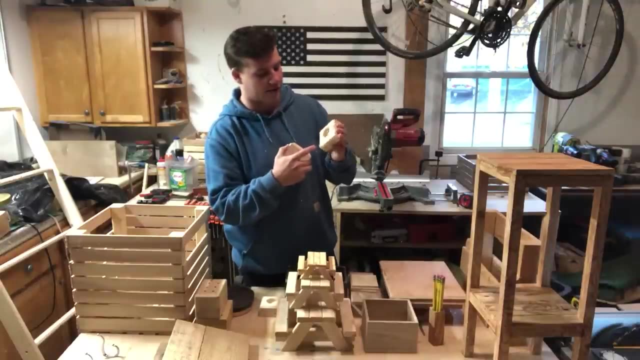 them here with me anymore. So that's it for those. Next moving on, we've got candle holders. Candle holders are great because you know they're easy to make. These are just 2x4s, and then you use a router on the edges, do something fancy And then you all you need is a one and a half inch. 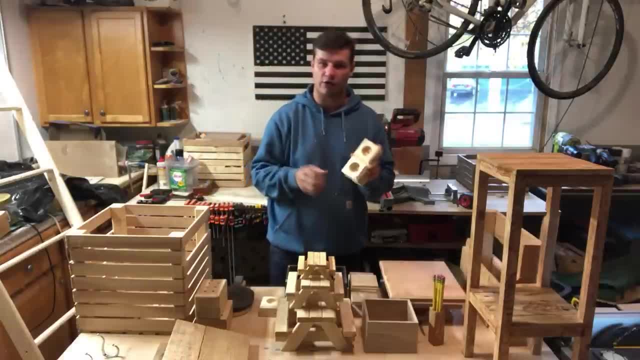 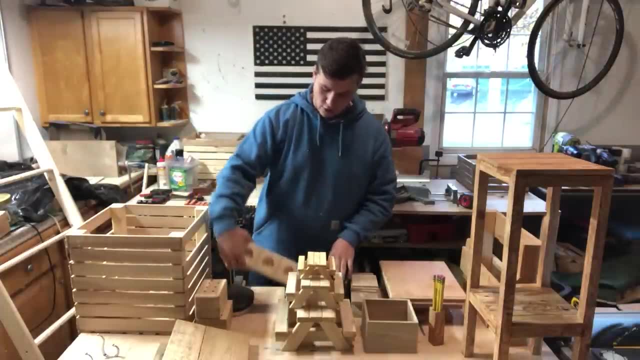 drill bit to go in there and that's the size of a regular, just little candle. So those are great for your dining room table, family room table, stuff like that. And then we've got another candle holder, but this one's got four areas for candles there. You see some nice centerpiece type. 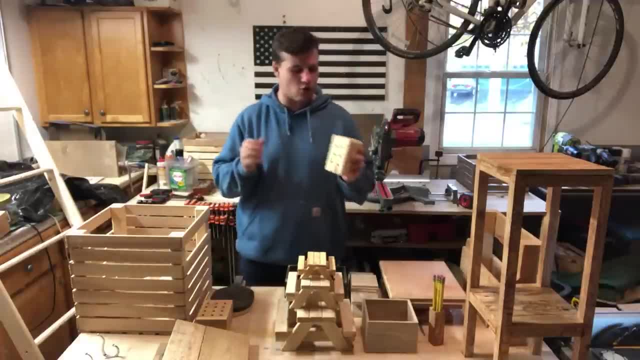 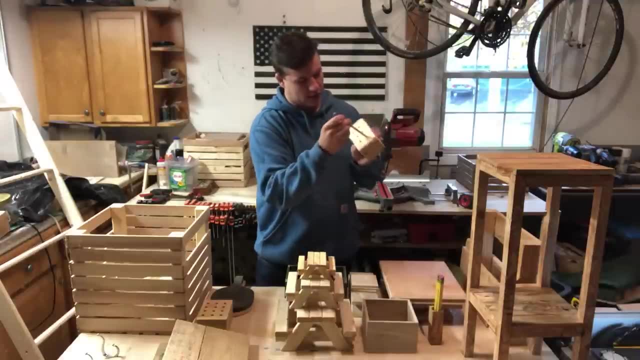 thing. So that's another great one. Then we've got a few different types of pencil holders, Again just 2x4s. Cut six holes in it with a little drill Drill, basically as big as a pencil Fits in, just like that. Really nice. And then round all the edges. And then we've got another, another pencil. 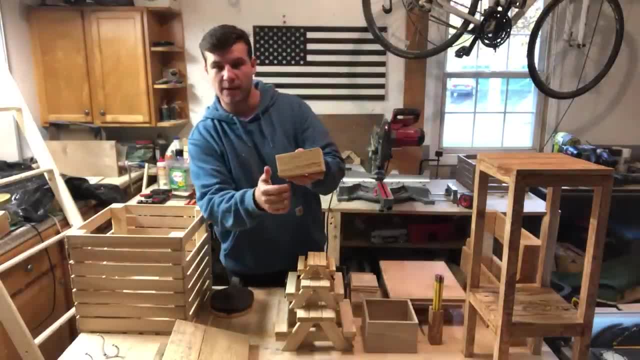 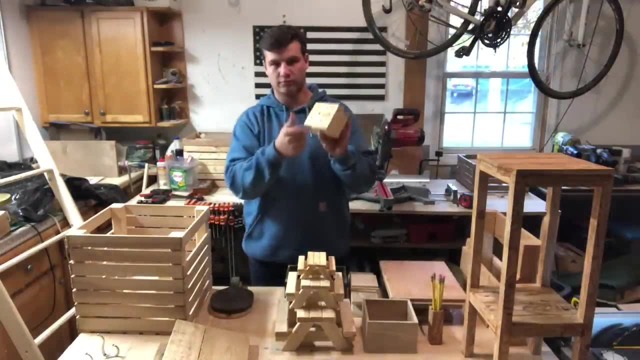 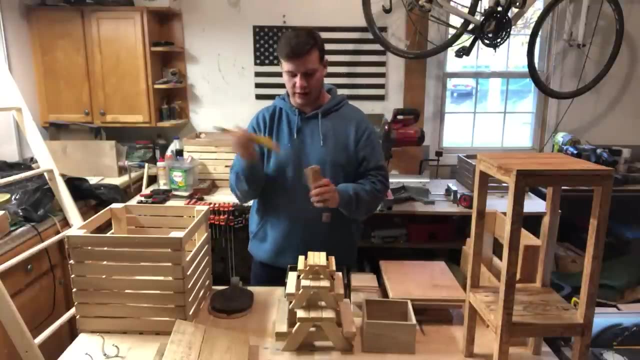 holder, but this one is plywood. So you, you got the nice grain pattern, the end grain pattern going on the top Again, perfect for fitting pencils. We have another pencil holder, which is just a really small one for the desk. I actually really like these Again. piece of 2x4 that I cut in half. 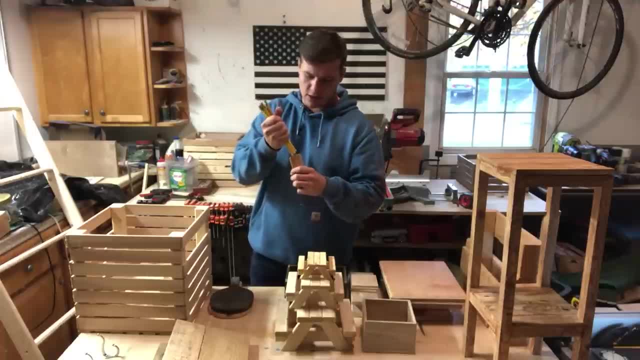 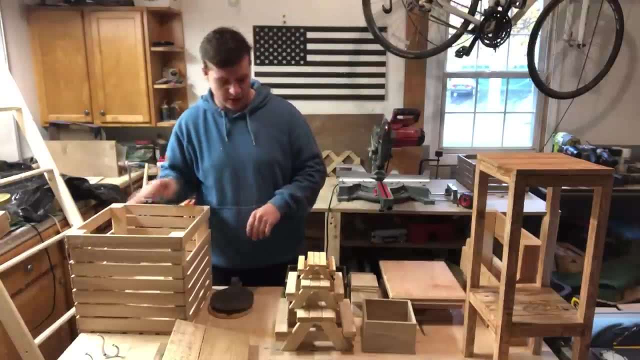 and then I just drilled a one inch thick hole in the middle And you know you can fit like seven pencils in there or something. So I really like this one Very simple project. but I've made a ton of those and I give those out as gifts all the time. The next one is a box. You can never go. 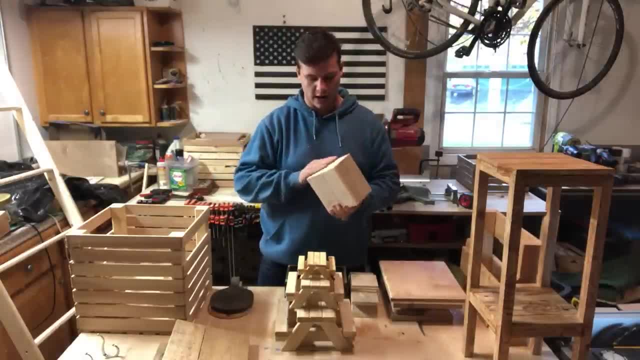 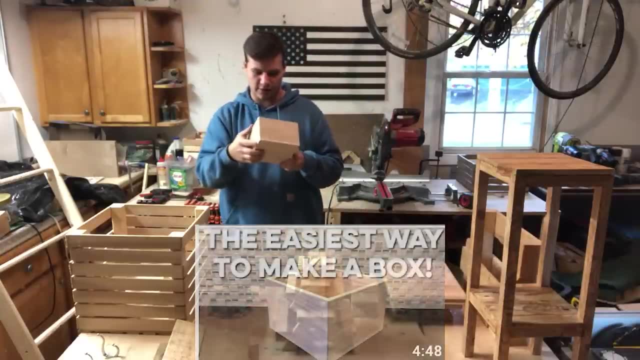 wrong with boxes, Gift boxes? I've made a ton of these, giving them away. This one, um, I made a video on how to make so that'll be in this corner or that corner, I don't know what corner, but John put that in, Thank you. Next we've. 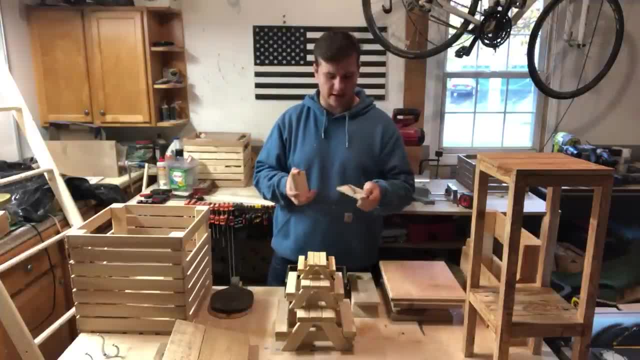 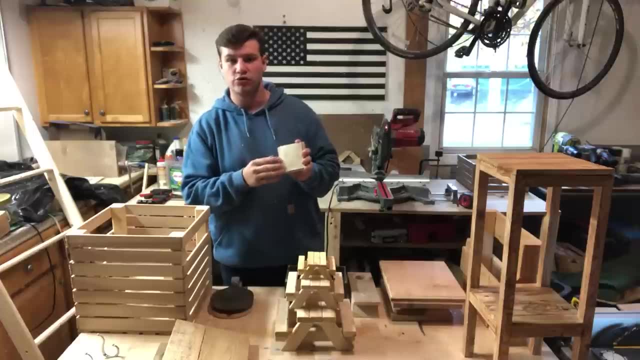 got coasters. Coasters are an obvious project that is so easy to make. These are just some scrap pieces of maple I had. They're about three and a half inches by three and a half inches. You can use a 2x4 to make these if you want to make them this size. but obviously, um, you know the maple. 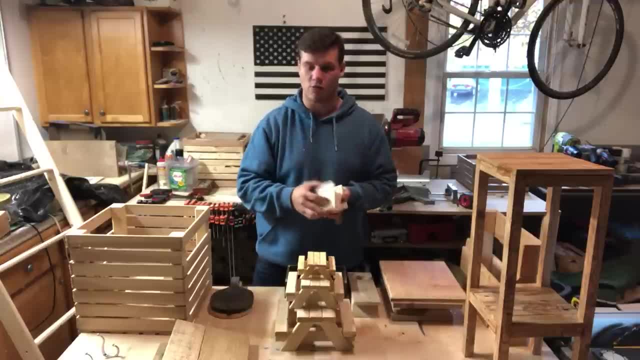 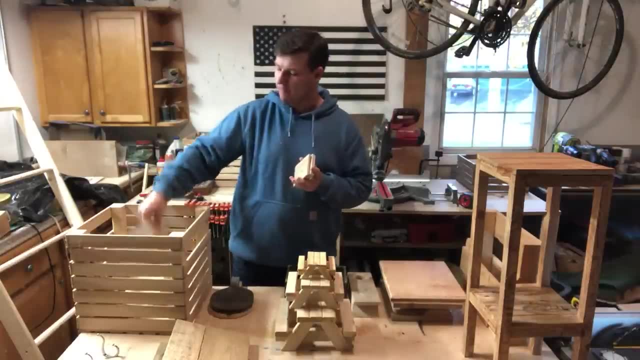 comes out looking really nice. All you have to do is cut it to the size you want, Put some poly on it, Sand. it Comes out looking great. If you're selling coasters, make a little box. Obviously this is too big, but make a little box with the same type of wood and just slide them. 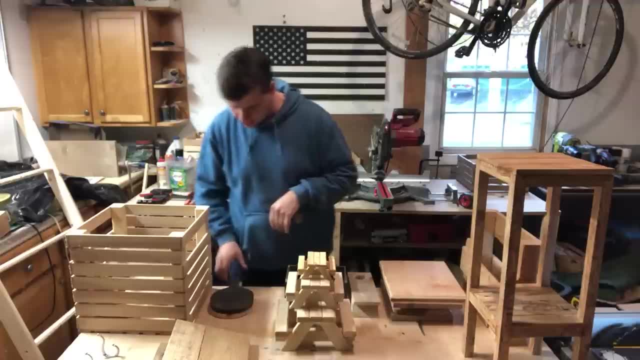 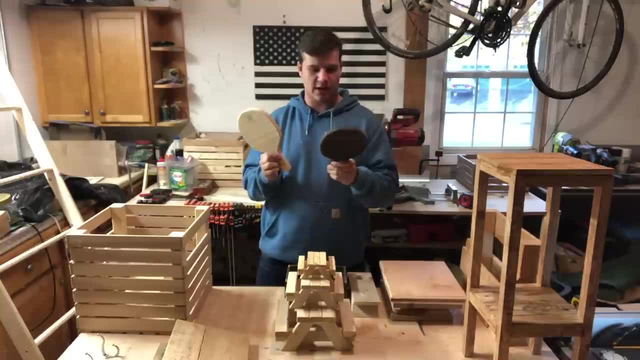 in there and you can sell them for a lot more money if you have that little box. Next, we have ping pong paddles. I was just screwing around one day and decided to trace one of my ping pong paddles and thought, hey, might as well make one of those. Um, so, these are cool. I decided to stay in. 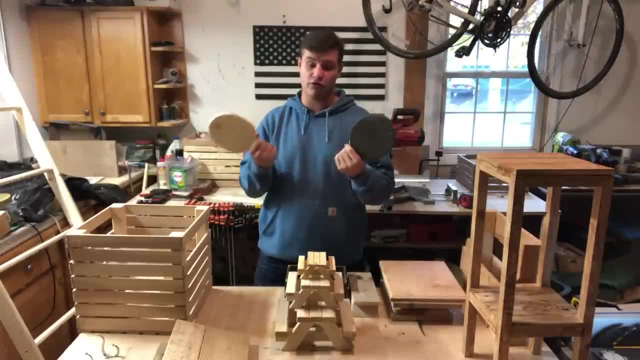 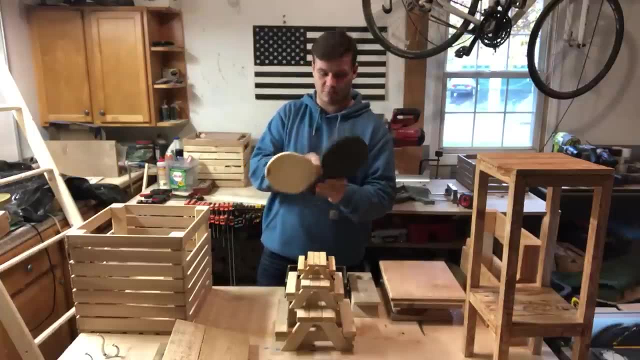 one and leave the other one there. So these are, they're usable. I played with them. I mean, you know they don't have any grip or anything, but they're fun to play with. These are going to help me segue to my next project. Um, like, if you put this together and you 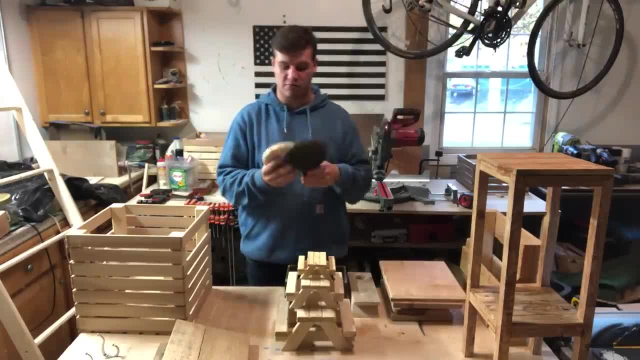 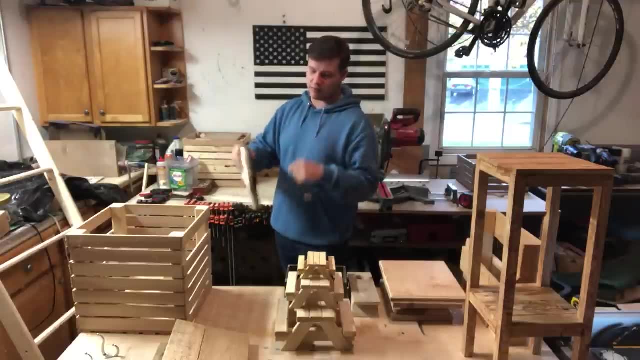 just glue these together or screw them together, Put them on the wall in your basement near your ping pong table, where mine is. That can be wall art, and I'm going to go grab a piece of wall art now that is in my room. Okay, I just went and grabbed the art from my room While I was there. 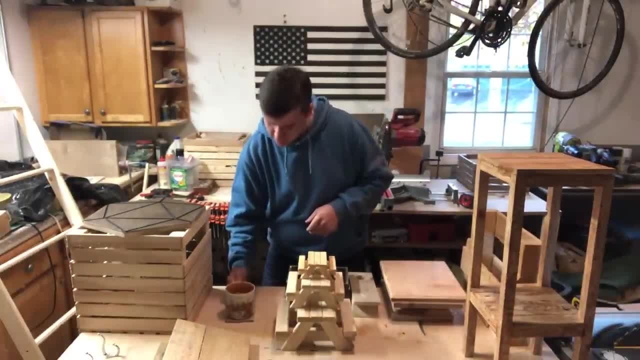 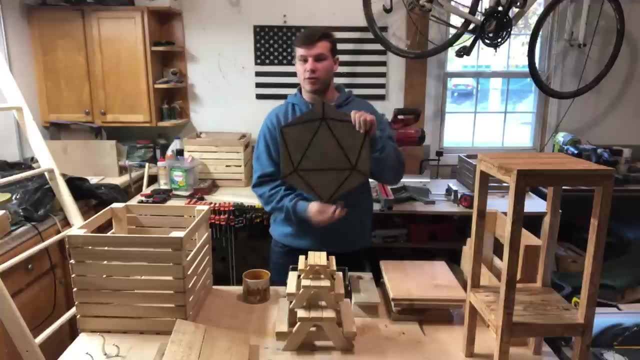 got myself a cup of coffee so I can show you how the coaster works. Look at that: The coaster works. You never would have thought, Never would have thought making a coaster yourself it would work, But it does. This is some of the wall art I made. This is the first. 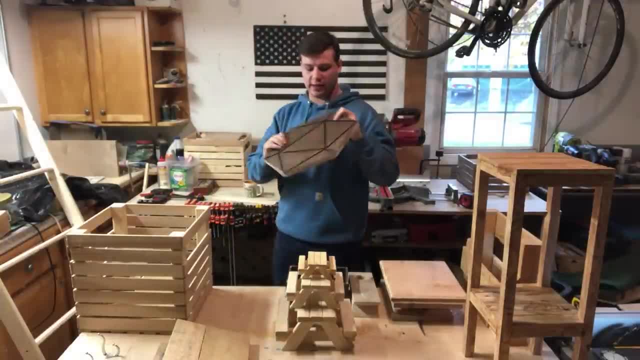 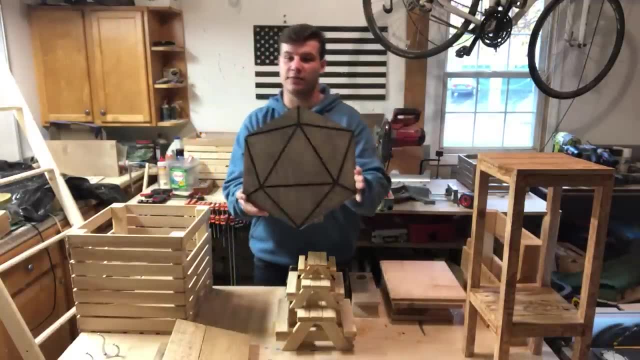 piece of wall art I made. So I really, um, I really like it. This is the Odessa logo. Um, I don't know if you know what Odessa is. It is a music group and they're my favorite group, So I decided to. 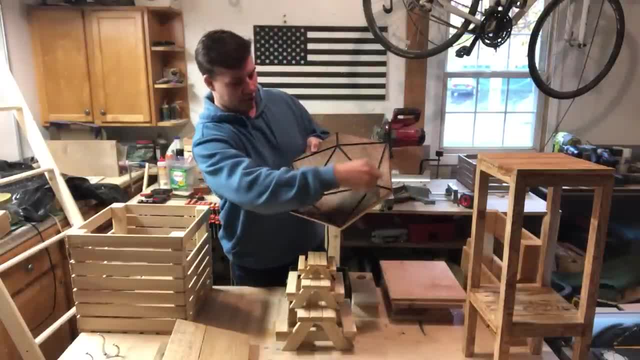 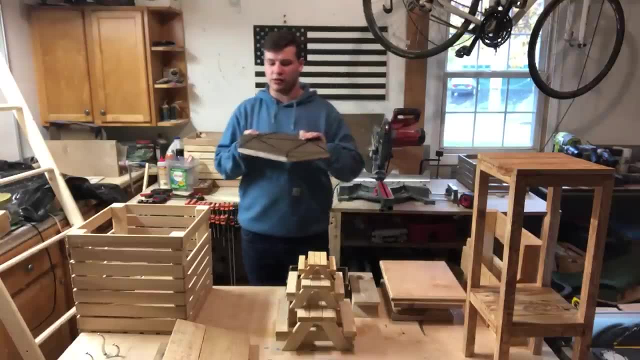 make the logo, and I actually used a router and I routed out these these black lines here. So wall art is something you don't really think about but you can make. I mean, it's it's still woodworking and it's still art. So I'm going to go grab a piece of wall art and I'm going to go grab a piece of 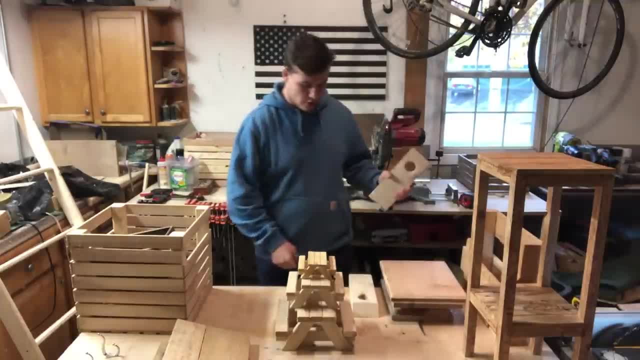 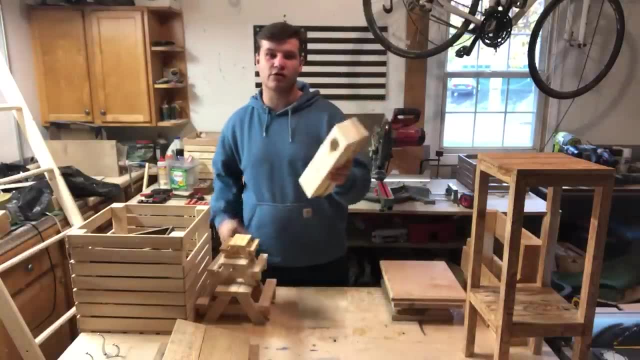 wall art. Next, we've got wine holders: Wine holders and floating wine holders. I have a video on how to make those in this corner, or that one. Uh, definitely check that video out, because these are great gifts to give. All you do is you place it down like that and then you put the wine bottle. 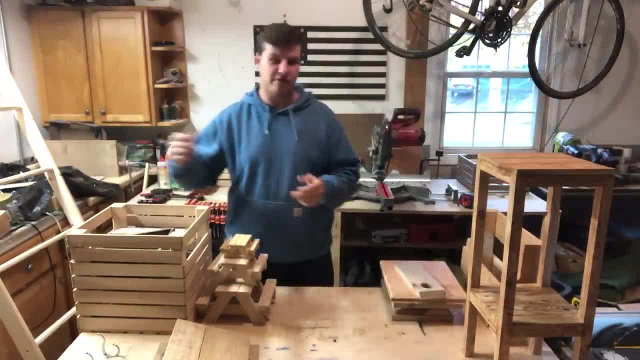 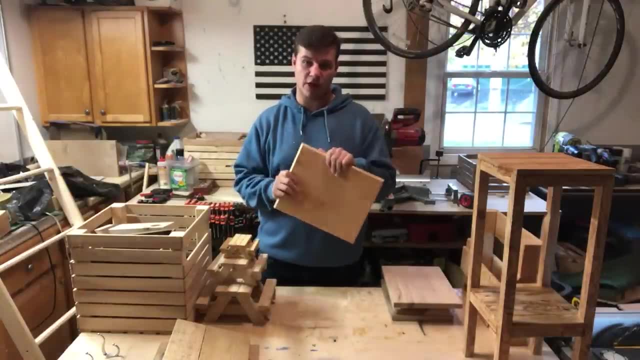 in this hole and it, uh, it floats. It's physics or something, I don't know. Moving on to another plywood project, This is a trivet or a hot plate. Do not use that as a cutting board, because plywood is not safe. Um. 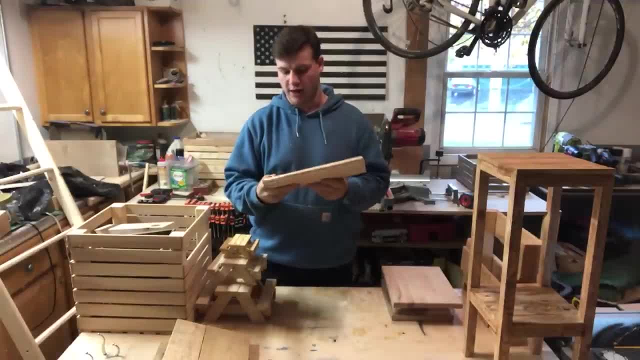 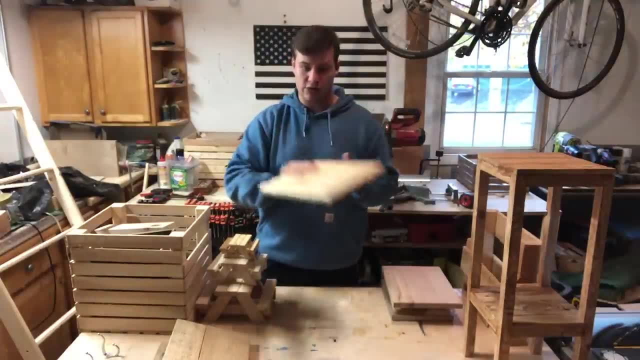 it's not food safe, but as a hot plate, go for it. So what I did is I had some leftover plywood so I just I routed the edges and then I poly the top and really made the grain pop out. So then you just place it down on your table and it looks nice and then you can put hot dishes on it and 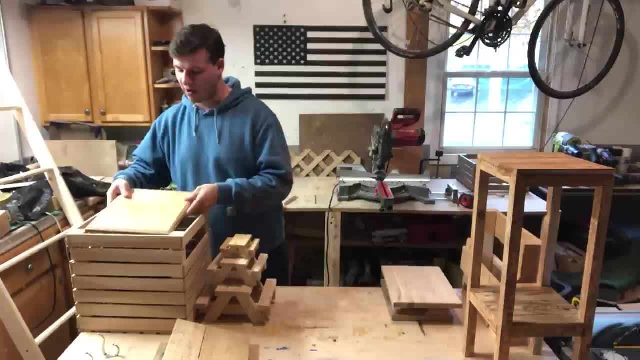 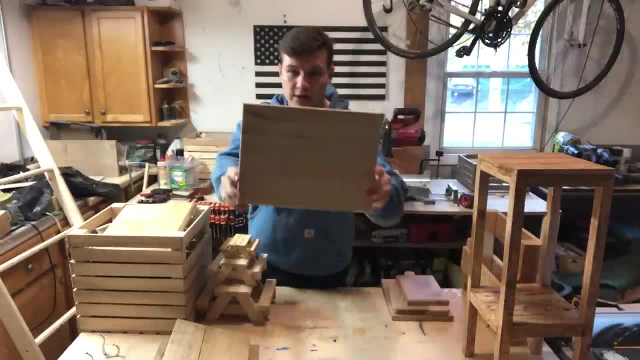 it's not going to burn it or anything. So trivets- Another great scrap project. Then we've got the cutting board, The classic cutting board. uh, with different pieces of wood. These were from a few different types of maple. there I have a video: how to make this exact cutting board actually. 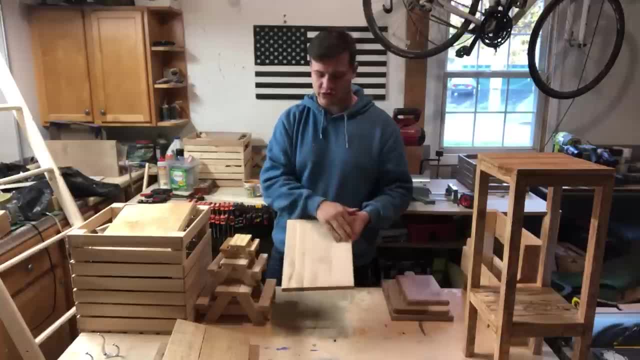 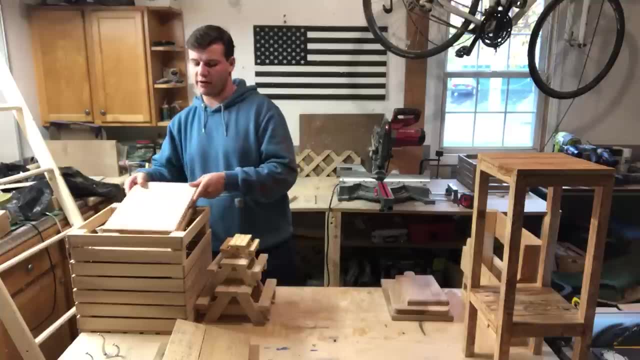 I have a video on my channel, so check that out in one of the corners. So this is just your classic cutting board, where you got a bunch of strips and you just glue them together. And if you don't have a planer, even better, because that's what that video is about: How to make it without a planer. 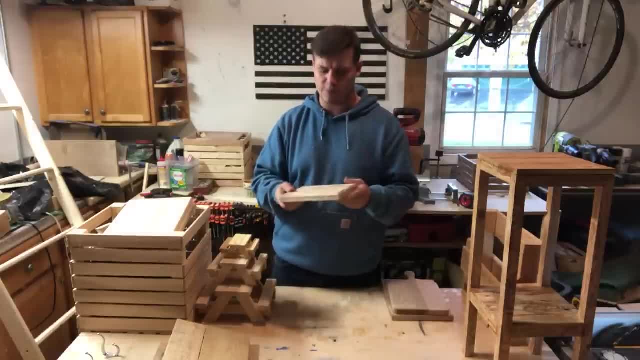 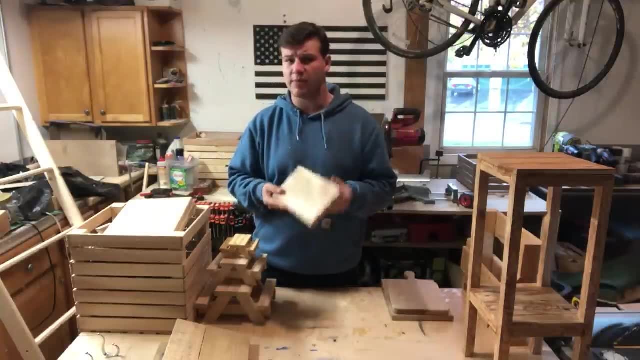 Another cutting board type thing. This is just a little cheese board I made, So it's a lot smaller. It was from another leftover piece of maple I didn't know what to do with. So basically the same as the trivet, although it's maple, so it is safe to eat on and and uh and you can cut things on it. 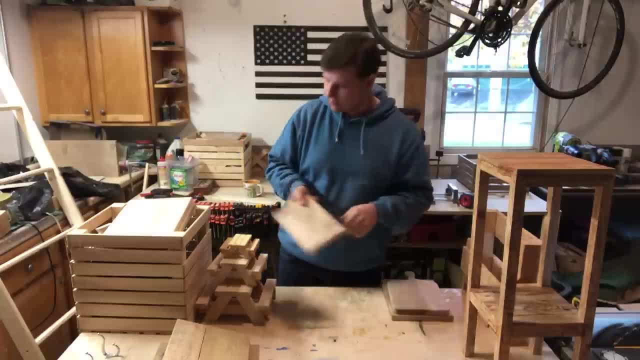 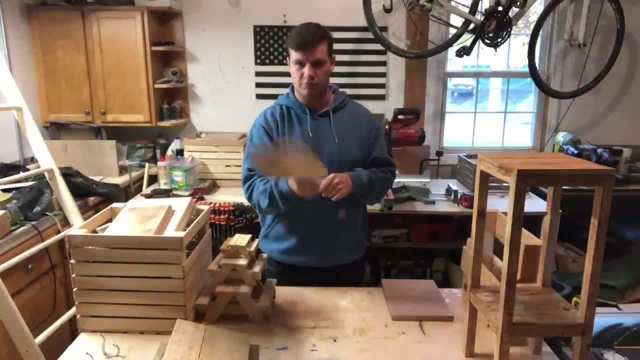 So there's a little cheese board on it So you can cut things on it. So there's a little cheeseboard- Uh, great for serving cheese. which brings me to my next project, because this is a cheese board or cutting board with a handle, which is the best for serving things. So you get your little charcuterie. 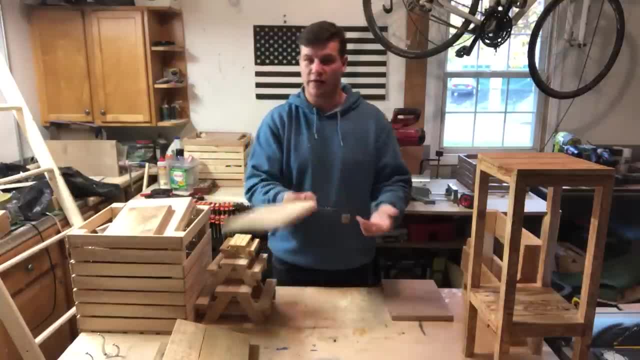 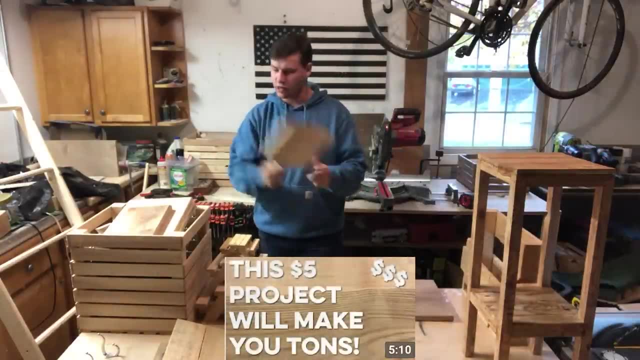 going Some, some prosciutto and cheese and crackers, and then you can just carry it like this. Really nice, Really easy. I have a video how to make this exact one on my channel as well. That'll be in one of the corners. Then we've got another cutting board, So I'm just going over all. 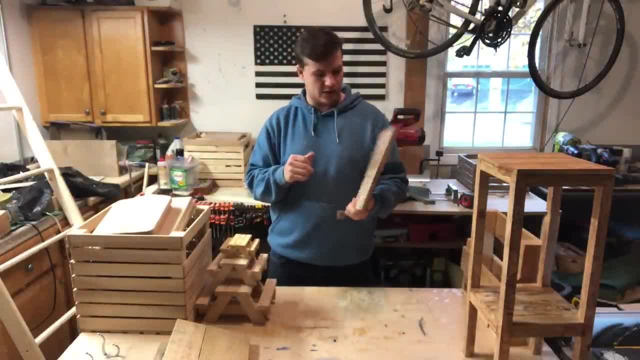 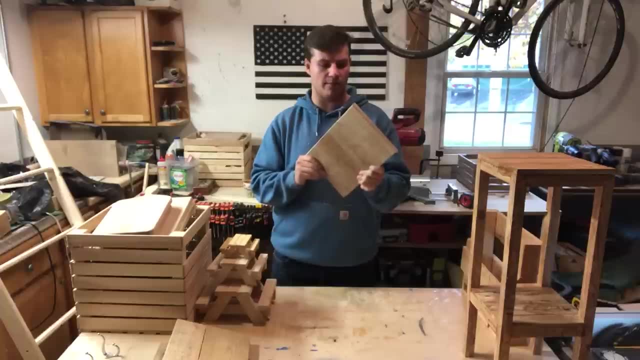 the different types of cutting boards. Um, I've got this is a cheese board. This is a cheese board, Another maple one. but I just glued two pieces of maple together And of course, with the cutting board, you always have to go over it with, uh, mineral oil, So it is food safe. So do that a few times. 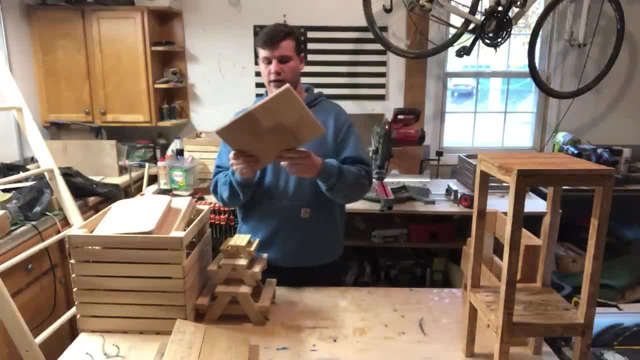 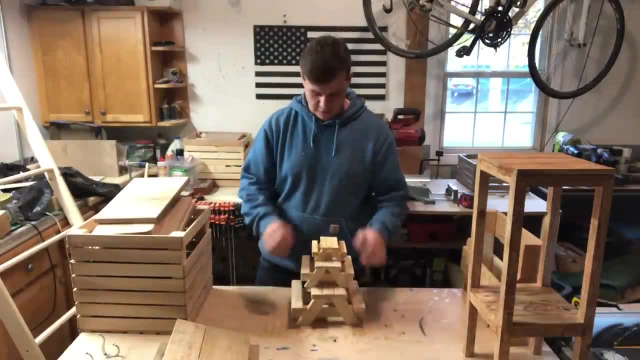 But yeah, this is just another cutting board where I just took two pieces of maple and I glued them together to make it a little bit bigger, But I think this one's really nice. Now we've got these little weird picnic tables that you've probably been looking at the whole time, So I have a video. 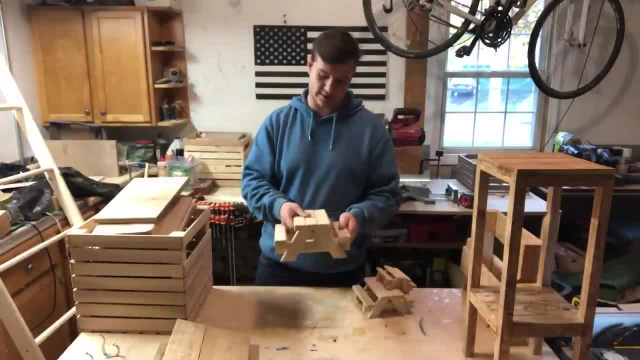 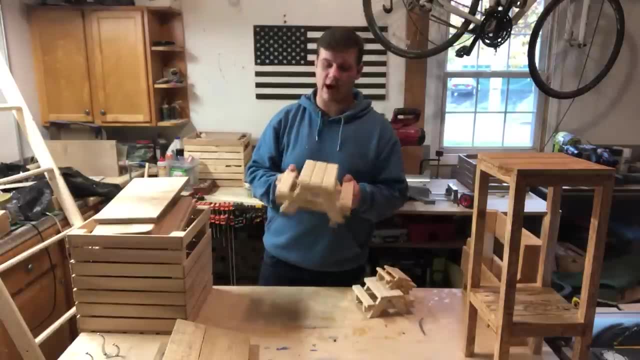 on how to make this big one. This is a squirrel picnic table. Uh, this is one of my best sellers as a video That will be also be in one of the corners. Squirrel picnic tables- A great, great project. Uh, they're a lot of fun to make And you can just put them outside or sell them. It's fun. 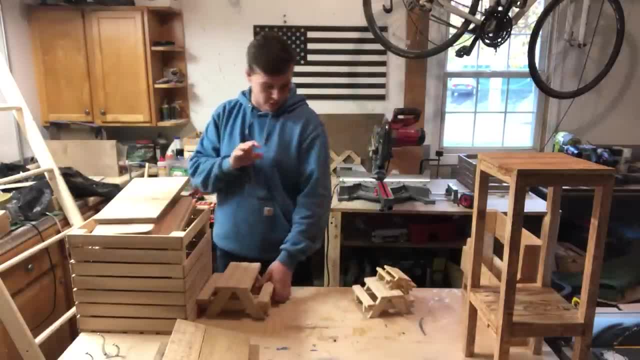 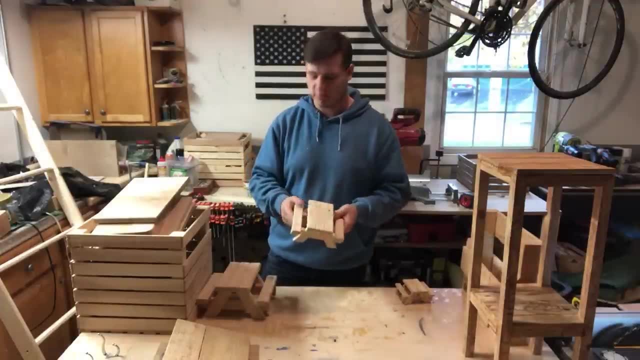 to watch the squirrels come and eat stuff off them. So squirrel picnic tables. And then we've got one a little bit smaller, which is a chipmunk picnic table, Because chipmunks are smaller. So you know, a chipmunk on this thing, it would, it would look weird, It would look weird. So 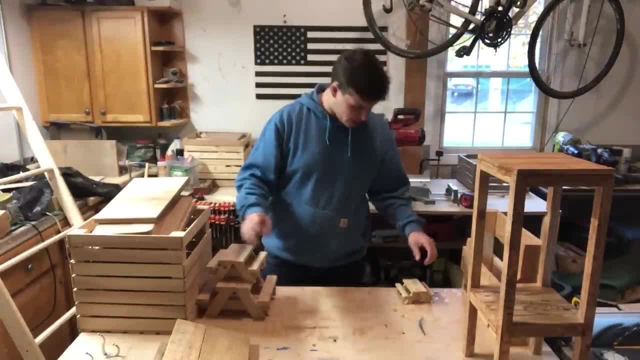 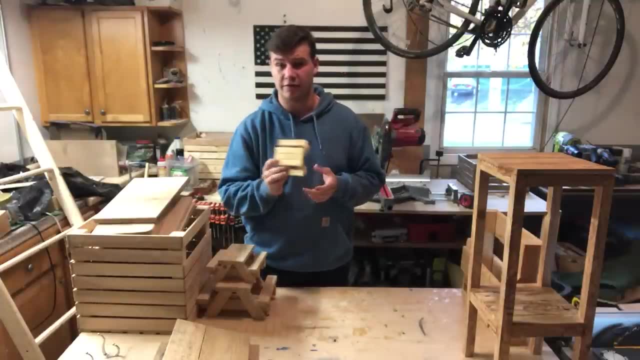 gotta make a smaller one for the chipmunks And then go even smaller for the hamsters. That toys are a great industry to get into as long as you make sure you have the right wood that is safe for, uh, the hamsters. So, like a hamster should not be chewing on this because it's pine, But if you just 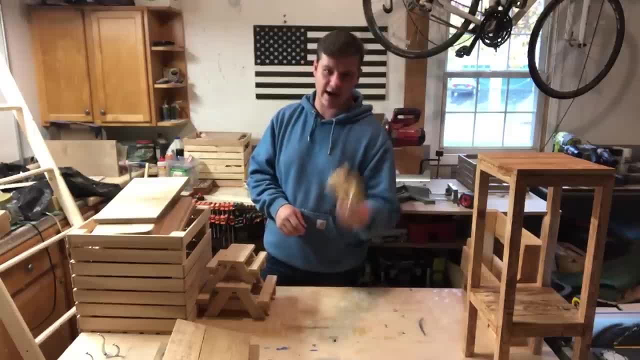 leave it in there and you put your their food on top of it. Then they come eat it and then you take it out once once they're done. Um, you know it's cute, It's fun. Now, moving on to this which I made. 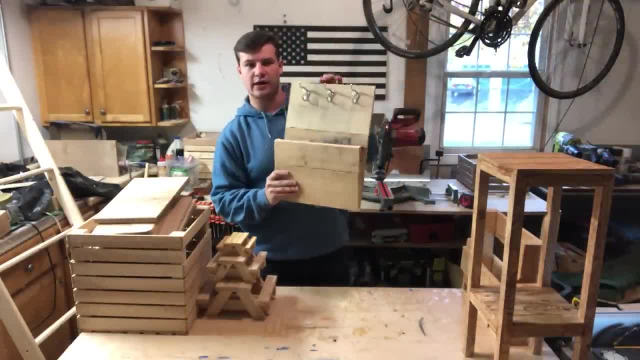 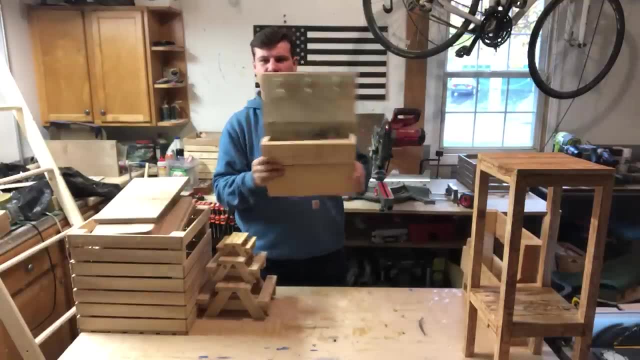 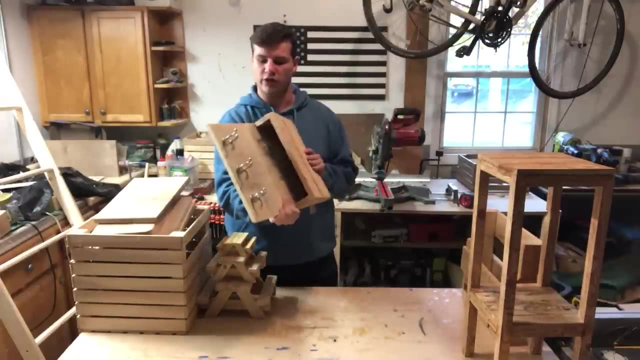 out of a- uh, a scrap pallet. Uh, it is a key holder, Key hook holder. You know you get the hooks there Also, just like in your laundry room or your mug room. You just put that right up there on the wall, Put the mail in, Put your keys up there. This one's really useful, Um, and I really like this one. 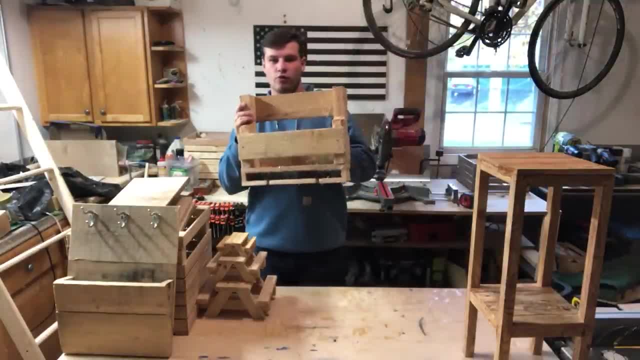 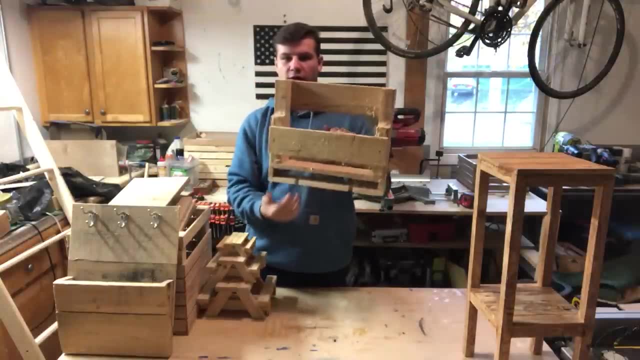 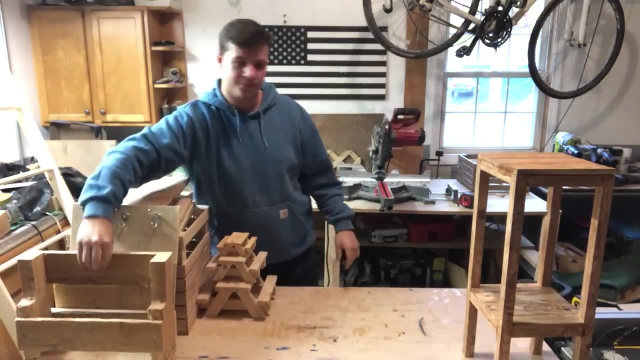 Another one we've got is the wine holder- Wine and glass holder- Which I also made out of a pallet. So here you've got the shelves for three bottles of wine there, And then you got two slits and the bottom there where you put wine glasses. You hang that up. That also will look nice Then we've got. 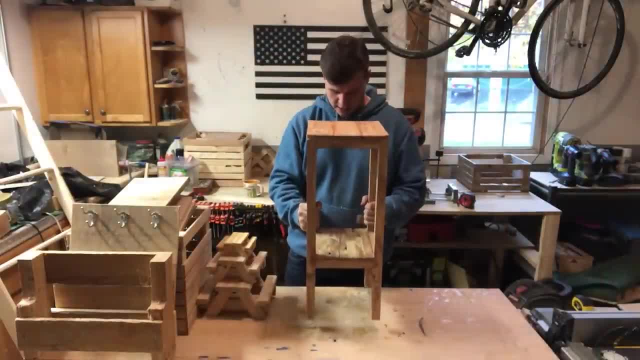 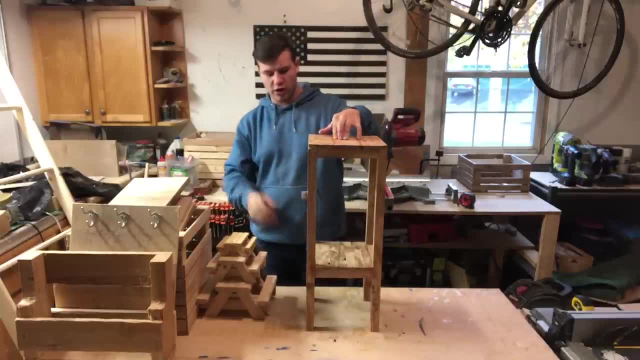 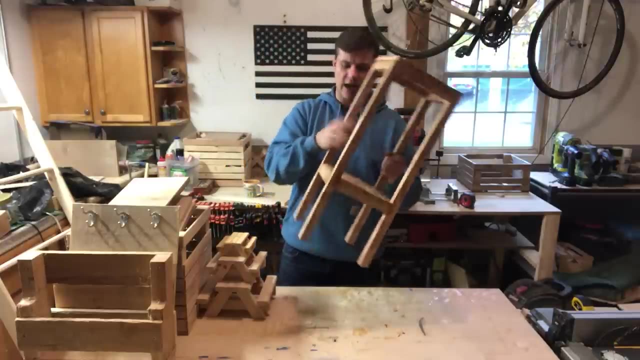 uh, end table, nightstand type thing that I made. Uh did another video on this one. I did, uh, the one two by four challenge. See, see what I can make out of one two by four. So this table is from one two by four. Uh, it's quite small but it's perfect for my bedroom. Sits right next to my bed, Has a little. 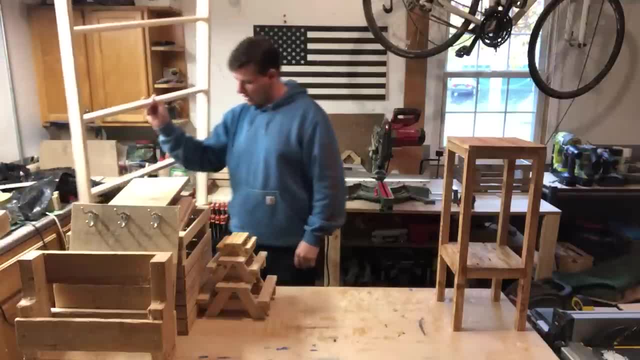 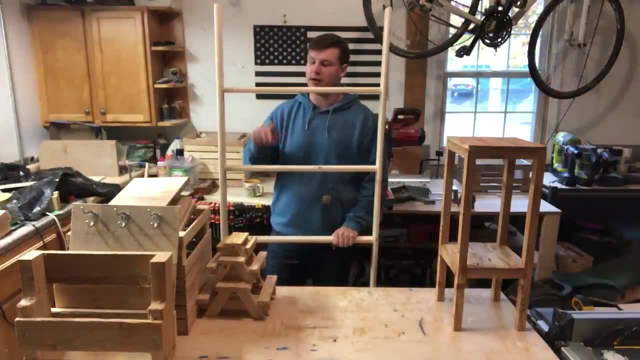 nightstand for water and my phone and stuff like that. Over here we've got a blanket ladder, Which I just did a video on How to make this. Blanket ladders are great And another one of my top sellers. People love blanket ladders or quilt ladders- Same thing. Um yeah, they're great. Five: 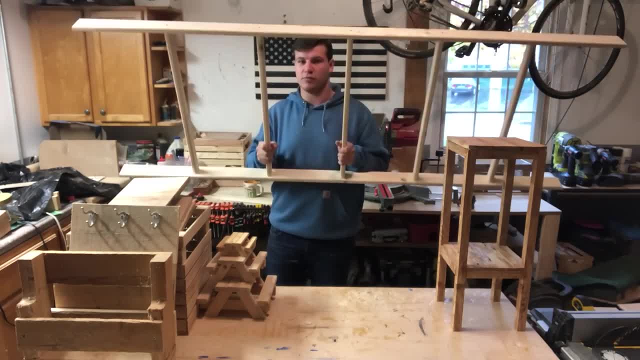 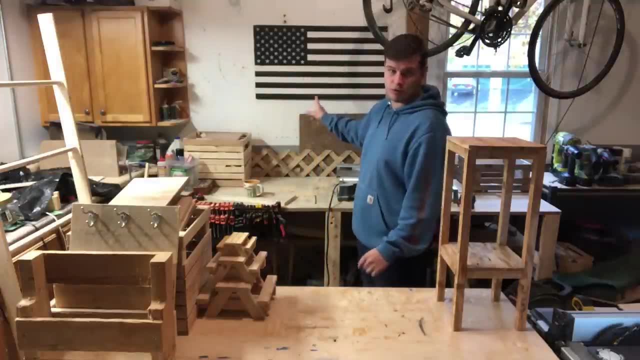 rungs for towels, blankets, quilts, anything like that. So blanket ladders are a really great project to do. I almost forgot. behind me we have a flag that I made. This also was from one, two by four. I'm big on making stuff from one, two by four. I guess I don't know what it is, But I also have 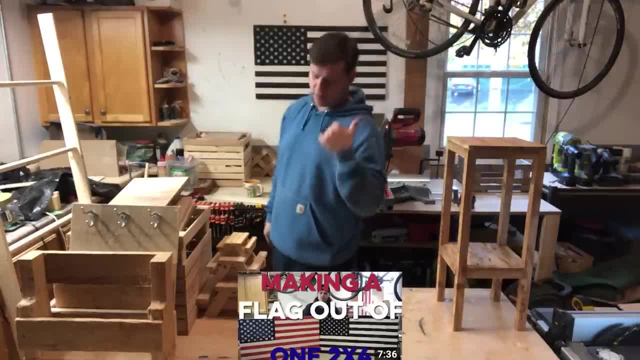 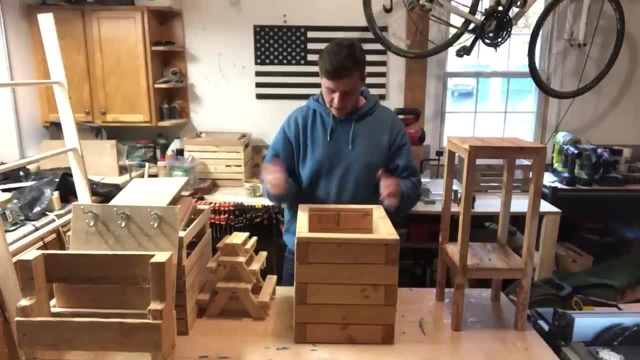 a video how to make this flag. Uh, and that is will also be in one of the corners. Really great project to sell. Super cool, I'm gonna make Came out looking really good. Next we have the garden box. Uh, or garden planter, I think it's. 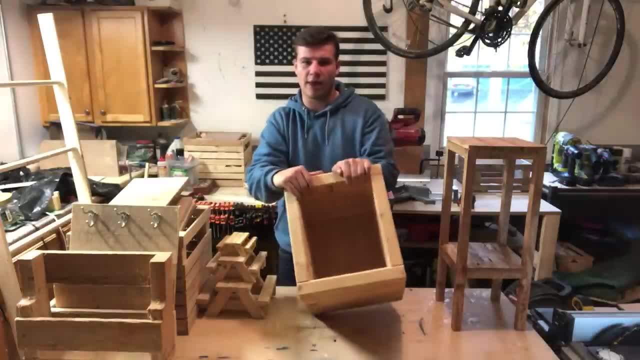 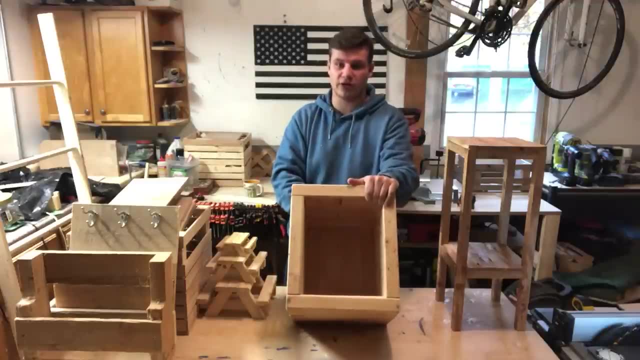 called. This is just made from some two by threes. I had, Um, and it is just a big, big old heavy box that you put dirt in And then you can put flowers and stuff in it. This is another great project, Uh, for outside for the summer. I know we're no longer in summer, But never, never, never, uh, never. 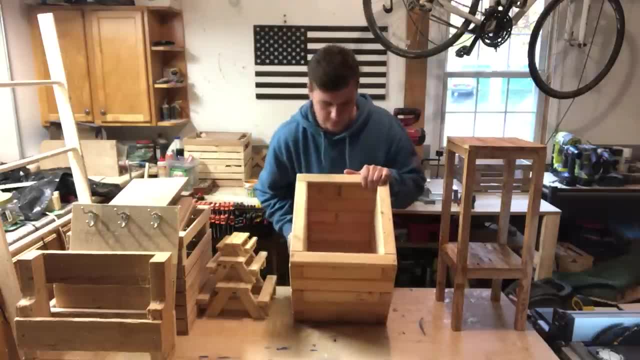 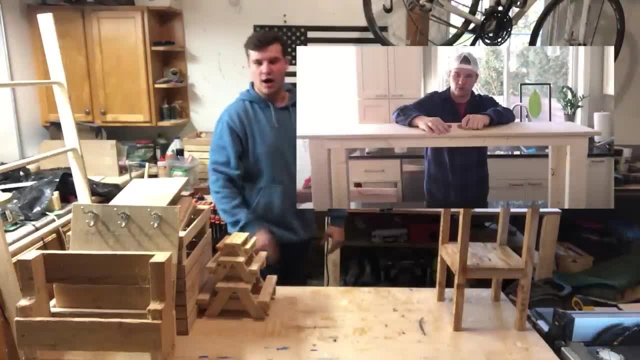 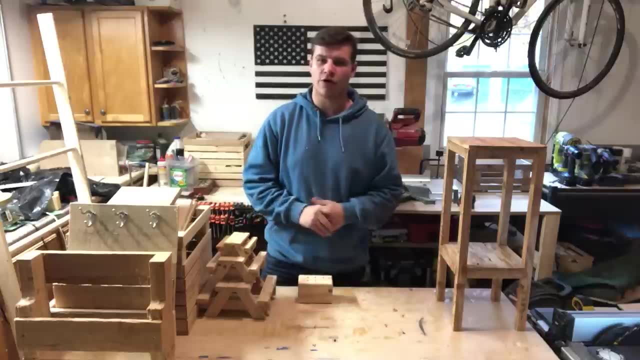 outdoor bench. Here's a photo of the outdoor bench. Uh, I did a video how to make that as well, which will also be in one of these corners if you want to learn how to make that. So another great project which is similar to this pencil holder I already showed you, is building blocks. People love. 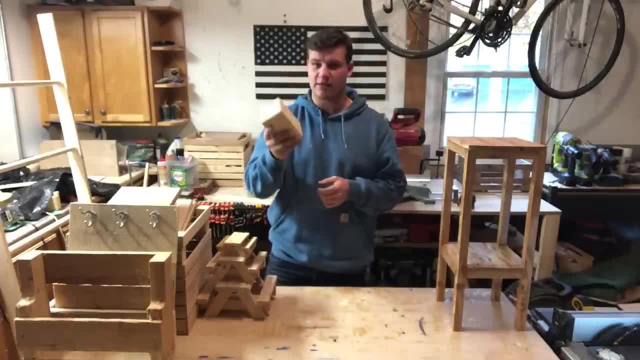 building blocks, uh, especially for kids. So if you just make this pencil holder just like this and then don't drill the holes in it, You've got yourself building blocks. If you make a bunch of different shapes and sizes, Those really sell well. I've seen a lot of people sell these on Etsy. I'm 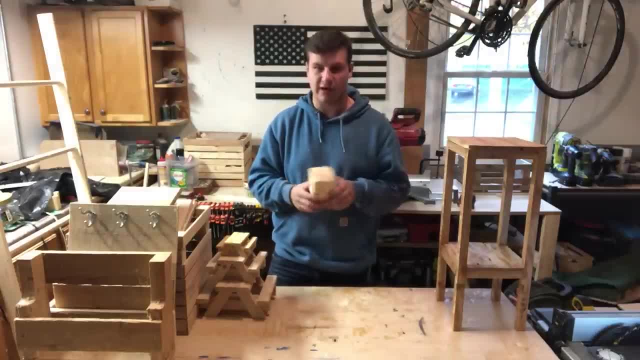 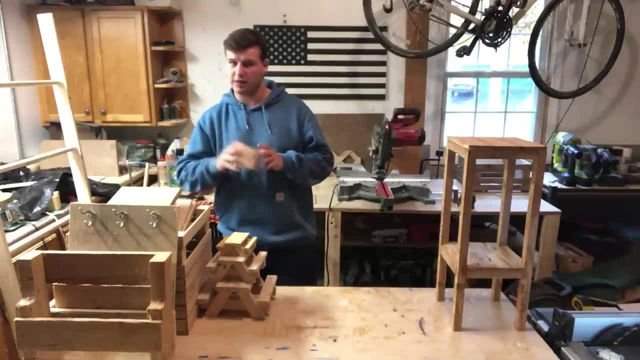 I've seen a lot of people sell these on Etsy. I'm I never really got into it just because you know it's not that fun, but you could definitely make some good money selling building blocks. So building blocks is another easy, easy project and you can make good money off that as well. The next project is a side table, which I also have a video. 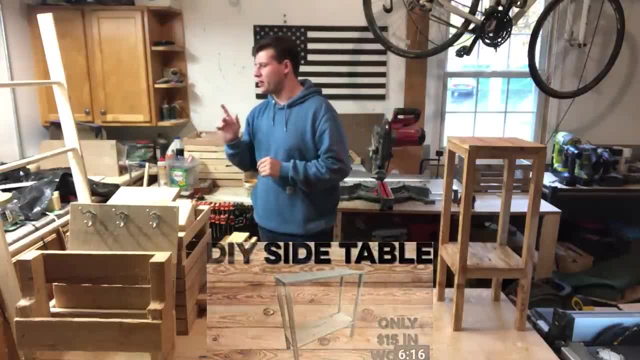 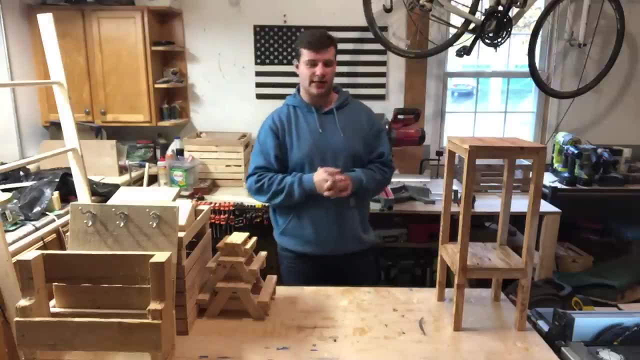 on how to build. It'll be in the corner as well. Um, side tables are great. Everyone needs a side table. That is also one of my best sellers. I don't make them anymore because I got bored of them, but side tables are great as well. The rest of these I don't have physically, so I'm just gonna. 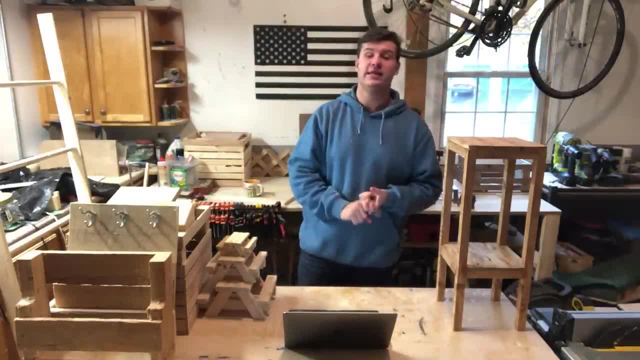 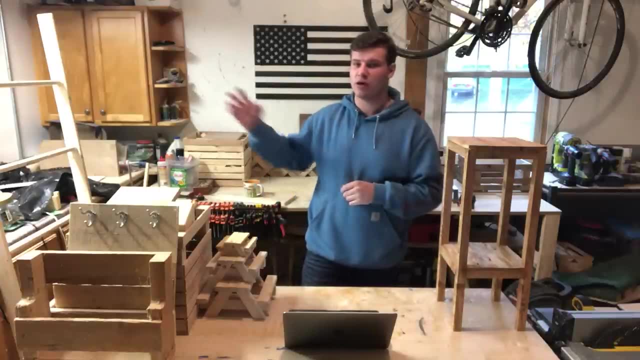 go over them and we'll we'll put pictures of them on the screen. Uh, TV remote holders. Just another little box, but you can put a line in the middle, um, and you can add little sections for the TV remotes. So here's a picture of that. Um, that is definitely a good one, Great gift as well. Beer. 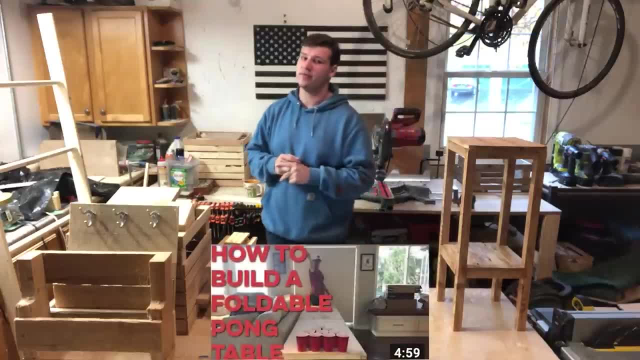 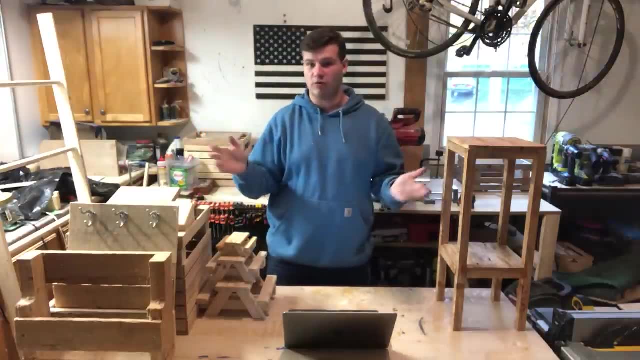 pong table. We have a video on that. You should definitely check that out. That's a great seller, especially if you live near a college. College kids love beer pong tables, So that's another great one. Coffee tables: How could I forget the coffee table? I've made a ton of coffee tables. I 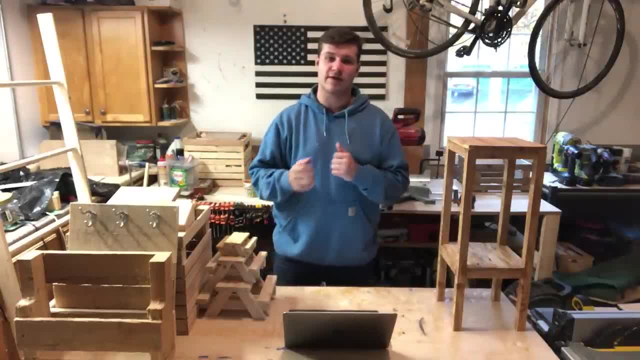 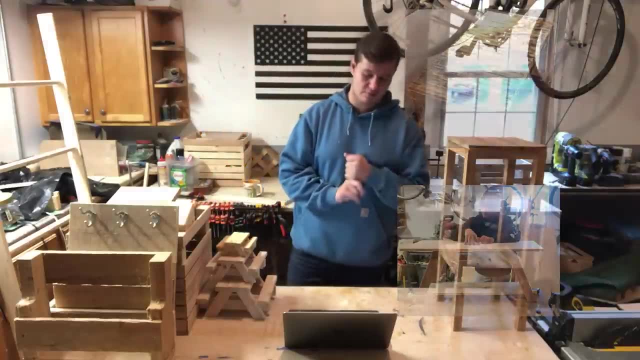 have other coffee table videos on my channel. I love making coffee tables- Definitely my favorite thing to make, Um, so here's a few pictures of some of the coffee tables I've made. Uh, so definitely, coffee tables are great. We got a hexagon shelf. That's just another wall hanging thing you can. 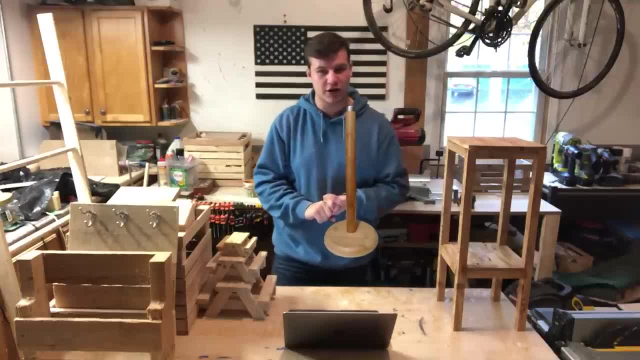 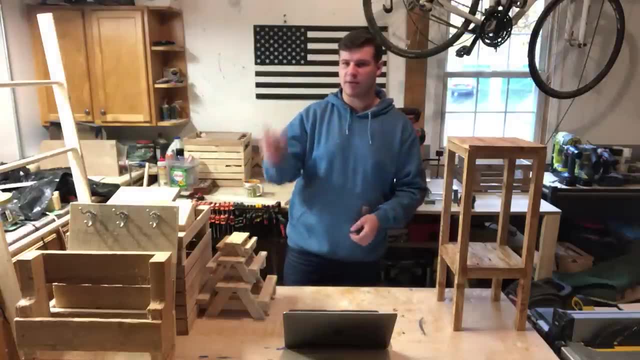 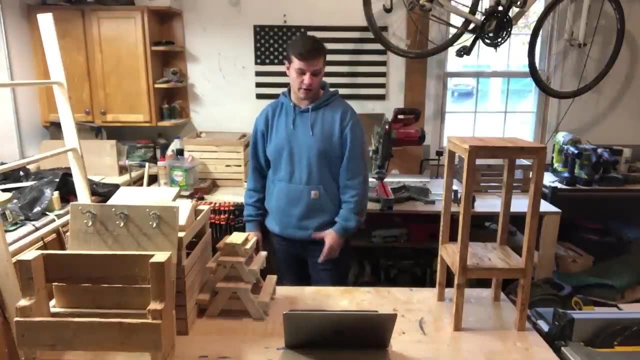 make. It's fairly easy. We've got paper towel holder, which I made once and I was actually kind of surprised by why I haven't done more of them. It's just a little simple paper towel holder, Piece of wood on top, Just a stick and you can put the paper towel right on there, Very easy. 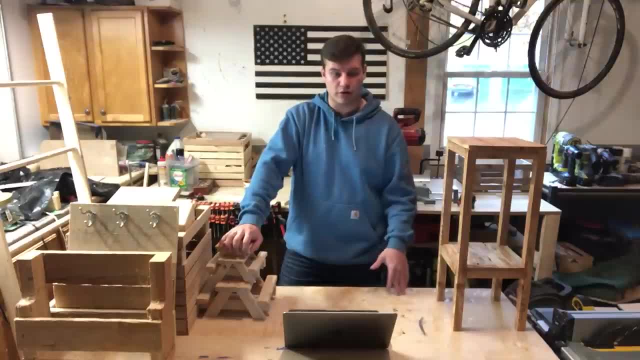 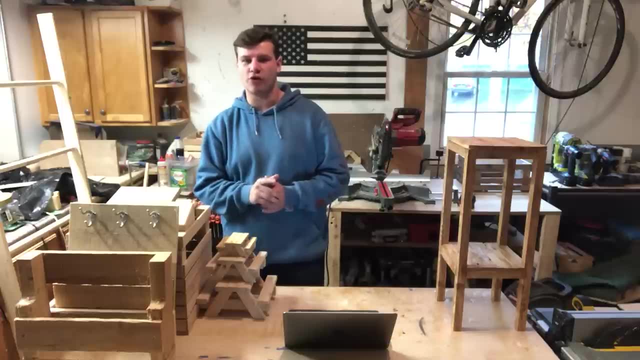 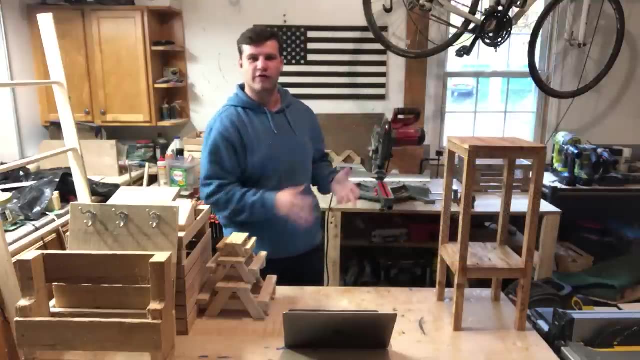 project that most people don't think about, That's for sure. Porn hole, Another great one, Should definitely, definitely good for the summers. One project that I've never made, but I see all the time, is this one picture of this couch hanging thing. It's like it's like it goes over the arm. 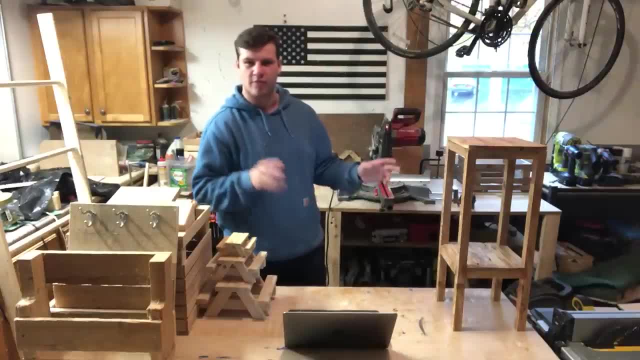 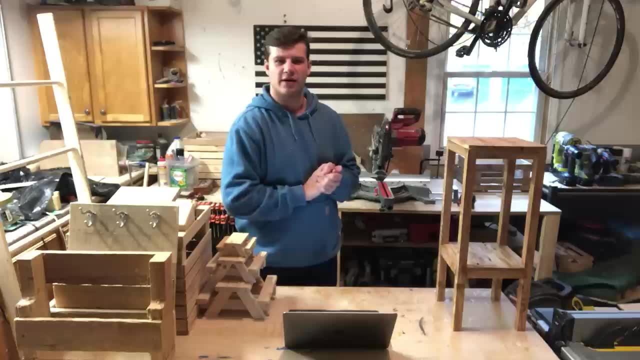 rest and you put your mug on it and that's got a little shelf. I think I can't exactly remember, but it looks like a good project to make. It looks like something I've never done before Anyone could use, and I think I'm going to make one of those soon. but since all the other videos,